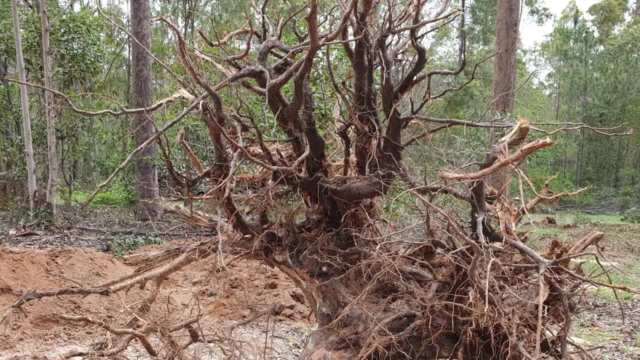 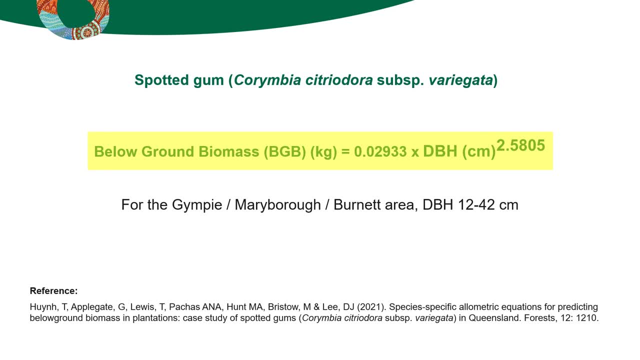 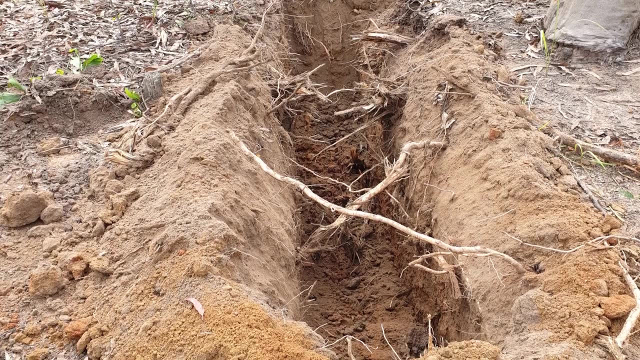 for particular species and locations. These are most accurate to use if available. This example shows a dry weight of spotted gum roots from plantations in South East Queensland. There are many other equations that have been developed for various species in various locations, and these 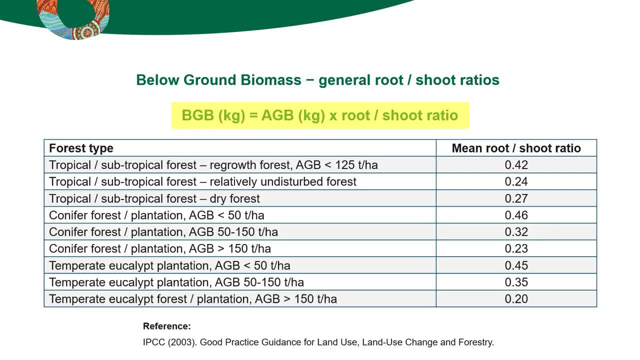 should be used if available. Otherwise, a general root-shoot ratio can be applied to the AGB of a forest. to estimate the BGB, These general ratios should only be used across a number of trees, such as a stratum or a forest, as they may not provide a very accurate estimate for individual trees. 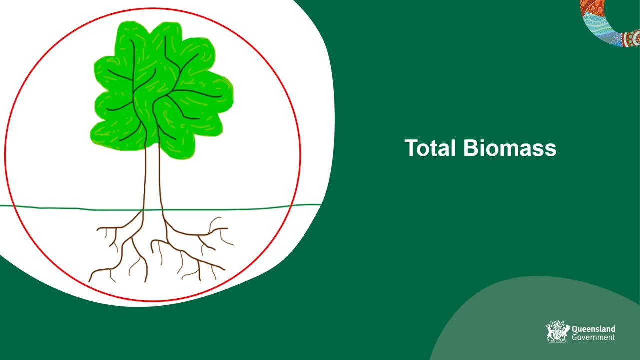 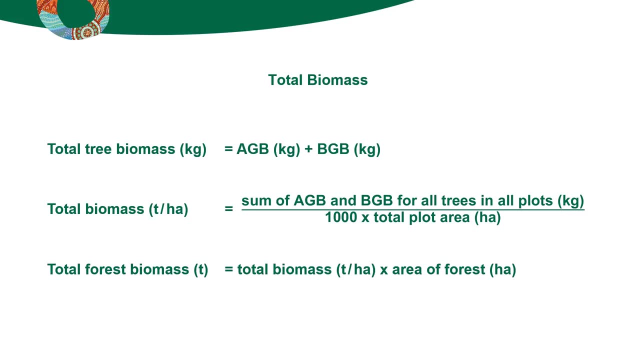 The total biomass is the sum of the AGB and the BGB, or the mass of all living parts of a tree or forest For an individual tree. once you have calculated the AGB and BGB values, they can be added together to give the total biomass in kilos For an entire forest or stratum. 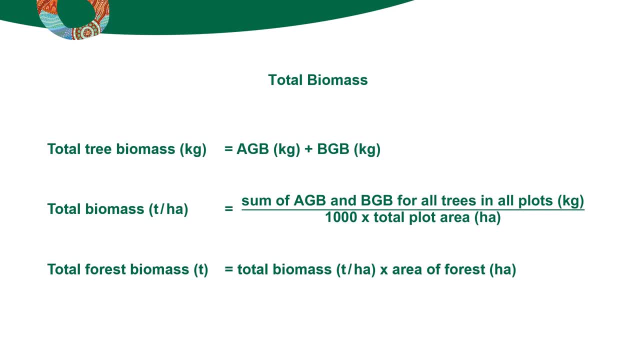 biomass is often expressed in tonnes of dry matter per hectare. So to calculate this figure, add the total biomass of all the trees in all plots in kilos, then divide by the total plot area and by thousand to convert from kilos to tonnes. The total forest biomass can also be expressed in tonnes. 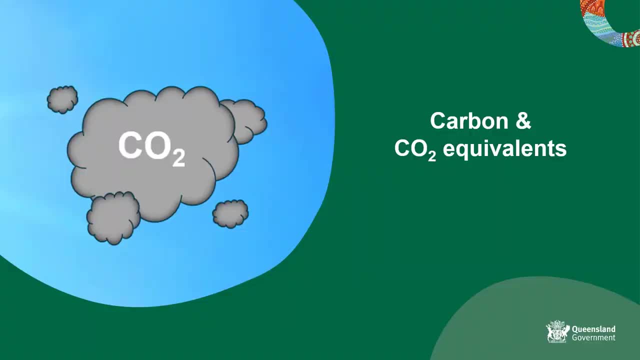 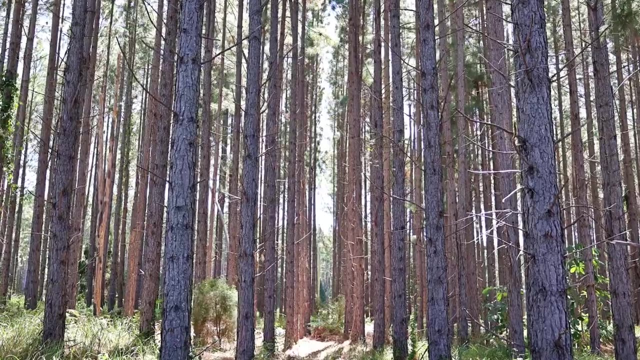 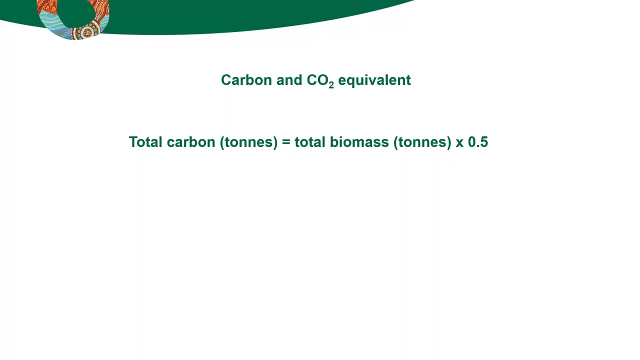 Calculating the carbon sequestered by a forest is an increasingly common reason to measure trees and forests. With the value of total forest biomass that you have calculated, it is an easy process to estimate both the carbon content and CO2 equivalent of your forest Total forest biomass. 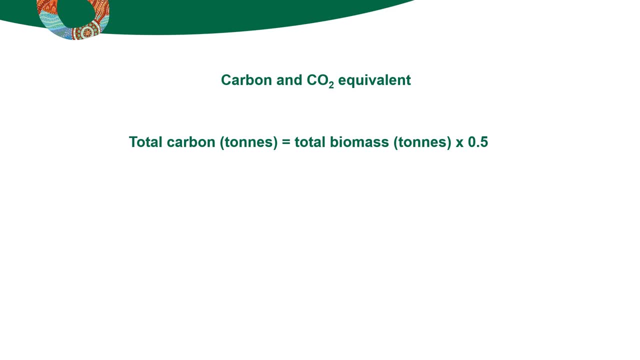 is converted to carbon by applying a carbon factor, which estimates the proportion of dry biomass that is carbon. Generally speaking, biomass is made up of around 50% carbon, so the carbon factor typically used is 0.5.. Greenhouse gas emissions are commonly reported as carbon dioxide equivalents. 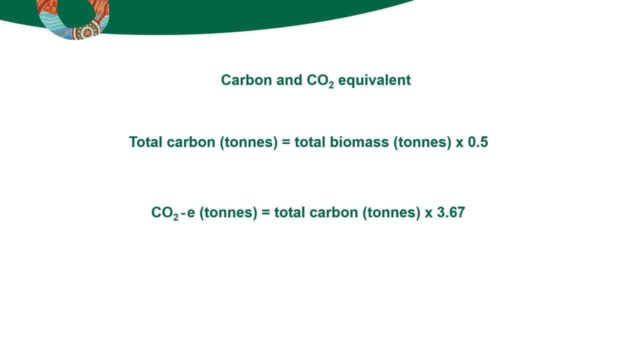 This measure allows a comparison of the impact of various greenhouse gases, such as methane or nitrous oxides, in relation to their degree of atmospheric warming potential. To convert total stand carbon to carbon dioxide equivalent, multiply by 3.67, which is the ratio of the weight of a molecule of carbon dioxide. 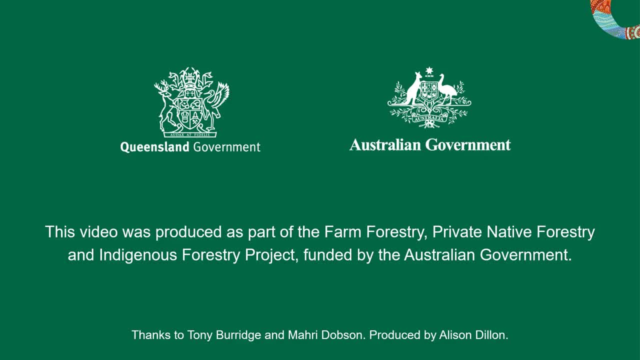 to the weight of an atom of carbon.